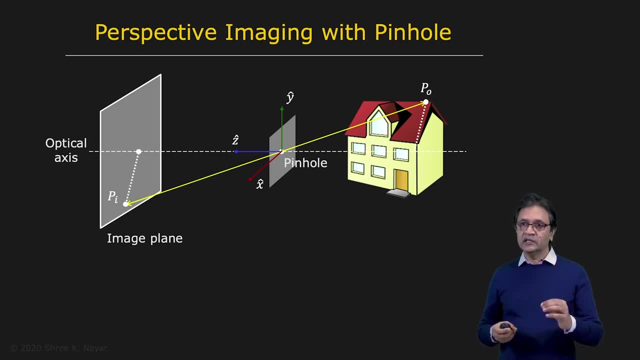 x, y, z, three-dimensional coordinate. And then we're going to write a coordinate frame placed at the pinhole, with the z-axis pointing along the optical axis. The optical axis, by the way, is the axis that is perpendicular to the image. 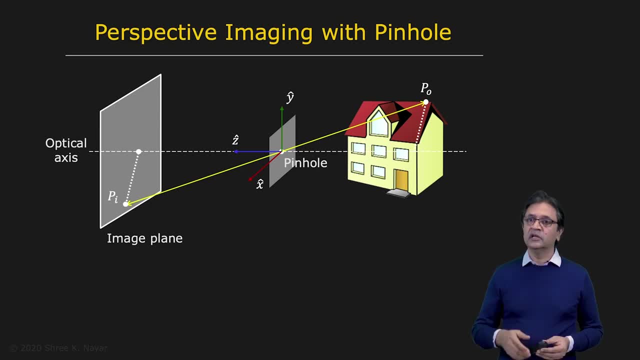 plane shown here as a dotted line. So the z-axis point towards the image plane and lies on the optical axis, And the distance between the pinhole and the image plane is called the effective focal length, and that's f. So now we can write the point P0. 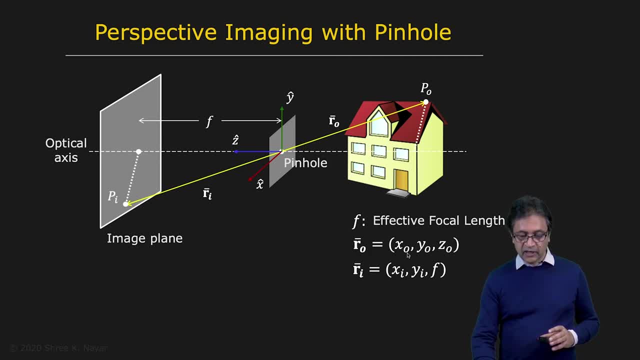 using the vector r0. And that has coordinates x0, y0, z0.. And its image can be denoted as ri, which has coordinates xi on the image plane yi, And the z-coordinate is going to be f. So, irrespective of where the point lies in three-dimensional scene, irrespective of its z, 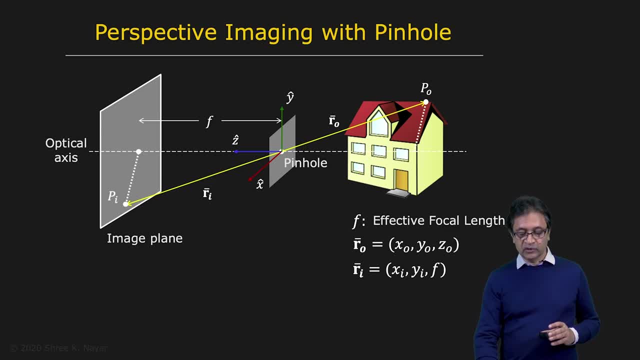 component, the z component on the image plane is always going to be f the effective focal length And at this point, to show final pitch for internships at all, that's actually going to flip 番 in lives of anybody except US debt. 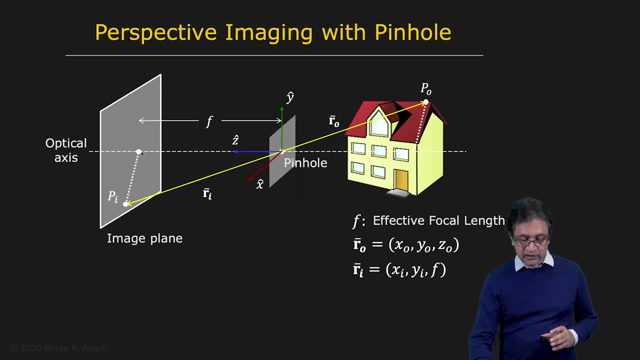 Now let's look at these two triangles right here: this one that I'm showing here and this triangle that's here on the back behind the pinhole. These are similar triangles And from these similar triangles you can write ri, the vector ri divided by f is equal to the vector. 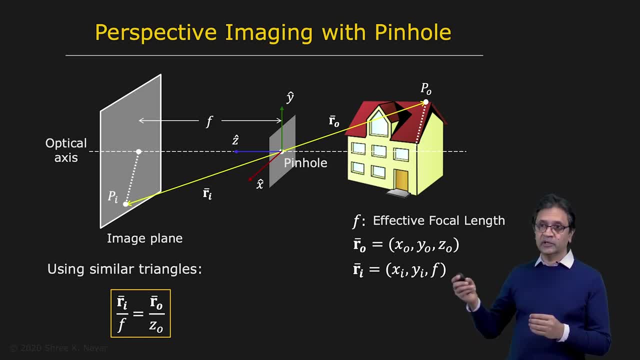 r0 divided by z0.. z0 is, by the way, the z-component of the three-dimensional point, the point in 3d. In other words, it's the depth of the point in 3D. And since ri and r0 are vectors, we 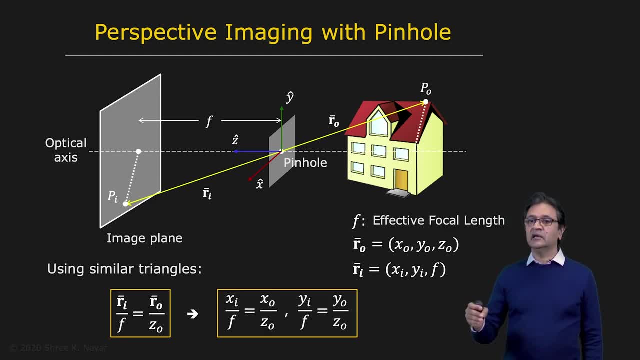 can break it down into its components and say xi by f is equal to x0 by z0, and yi by f is equal to y0 by z0.. These are the equations of perspective projection. Very simple equations but create some fairly non-intuitive effects in images. 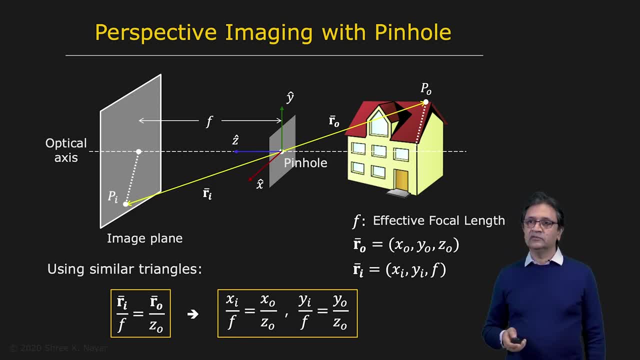 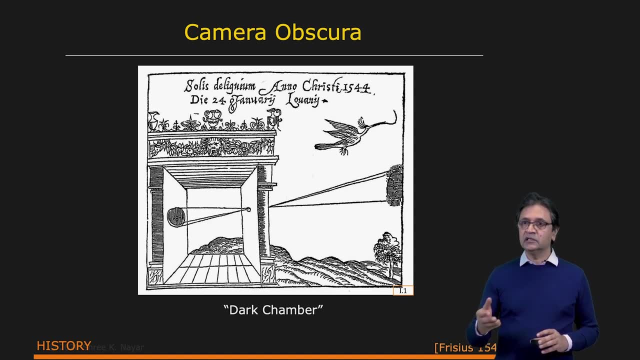 So this idea of pinhole projection and a pinhole camera actually dates back to 500 BC. There were Chinese philosophers who were writing about this concept way back then And then, somewhere around 1000 AD, the Arab physicist Al-Hazan. he wrote a book called. 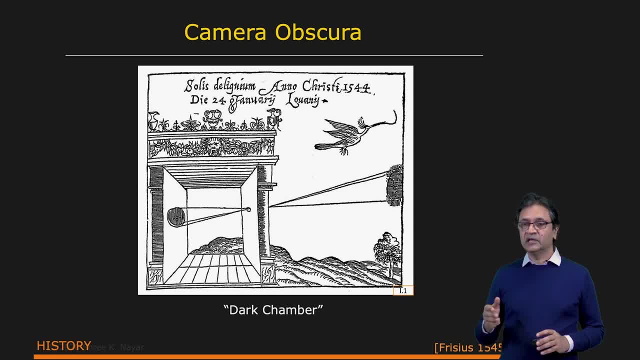 Kitab al-Manazir. It's actually one of the first optics books. He describes in great detail the concept of pinhole projection. He describes in great deal this concept of the pinhole camera And it's only in the 16th century that this concept actually. 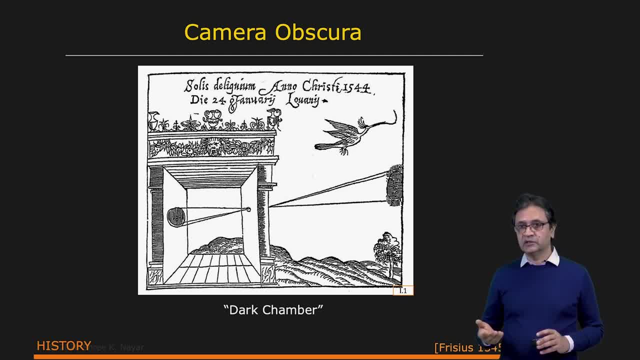 came to the West, It became very popular among artists, particularly as a tool for rendering accurate depictions of three-dimensional scenes. So here is a sketch by Gemma Frisius- It's a Dutch mathematician- where you can see that there is a wall with a little pinhole. 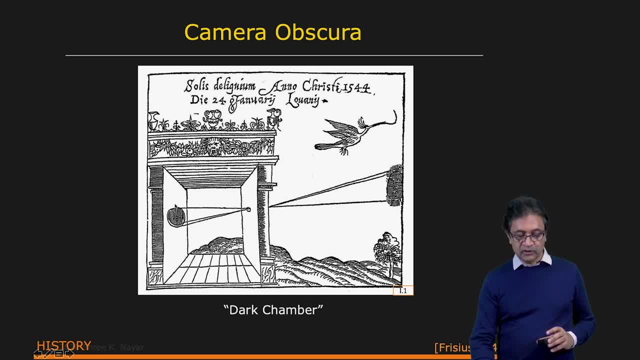 a little hole in the wall, and behind this wall is a second wall, And so the three-dimensional scene gets projected by this pinhole onto a two-dimensional image, And now you can imagine that an artist can walk up to this wall and sketch out a very accurate geometrical representation. 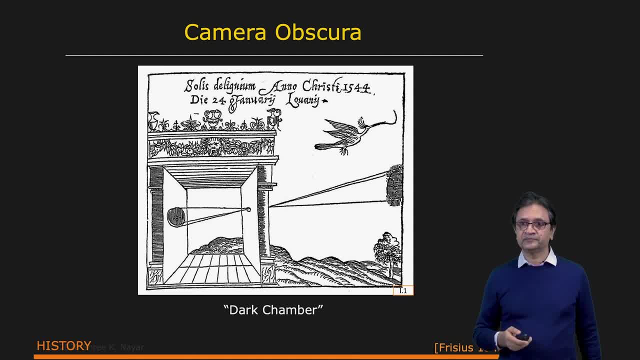 of the perspective, projection of the scene, a picture. By the way, this concept was called camera obscura, which in Latin means a dark chamber. Well, when it comes to the pinhole camera, as with many other things in life, nature got there first. 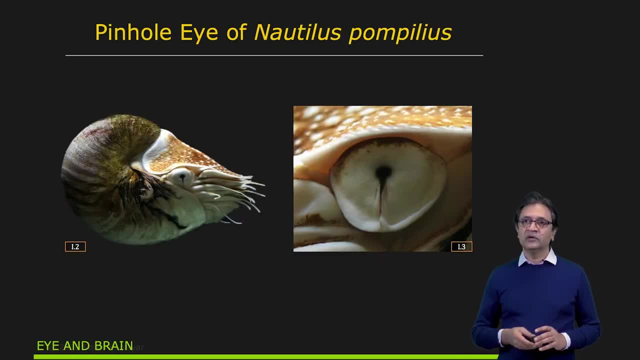 So here is an eye which is a pinhole eye In the case of this creature. this is a shelled sea creature called Nautilus pompilius. You can see that it has an eye right here and it has a fairly large pinhole which creates an image. 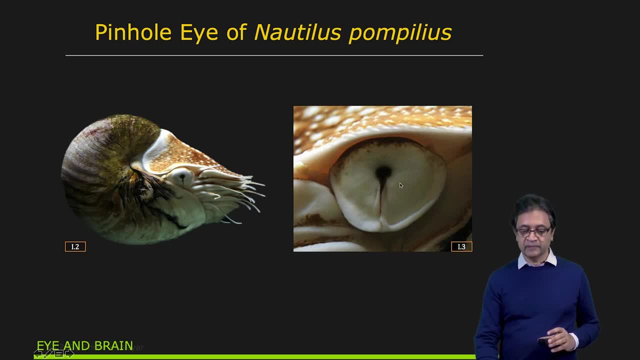 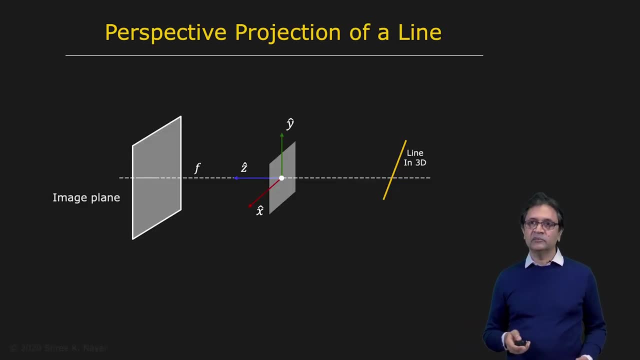 and there is no lens in this eye. All right, now let's take a look at some of the properties of perspective projection. The first one I want to talk about is: what is the perspective projection of a line in 3D? So here you see a line in 3D and you 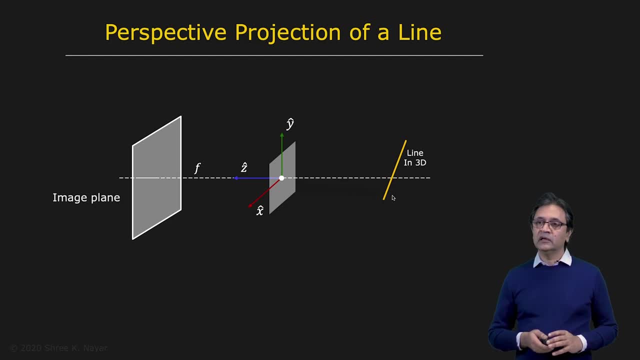 have your pinhole right here And we know that the line and the pinhole- that is a line and a point- define a plane in 3D And all the rays of light that pass through the pinhole lie on this plane. 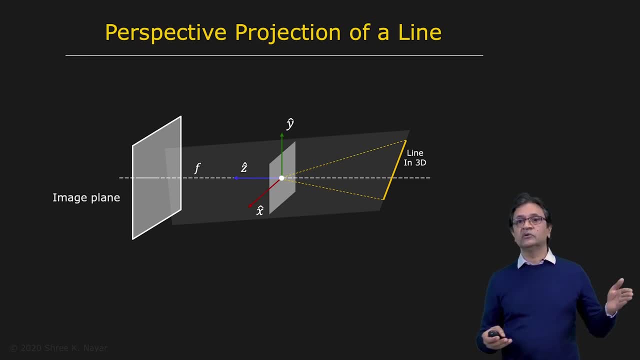 And, for that matter, all the rays of light that pass through the pinhole towards the image plane also should lie on this plane, And so the image of this 3D line on your 2D image must be the intersection, must lie at the intersection of this plane and the image plane. 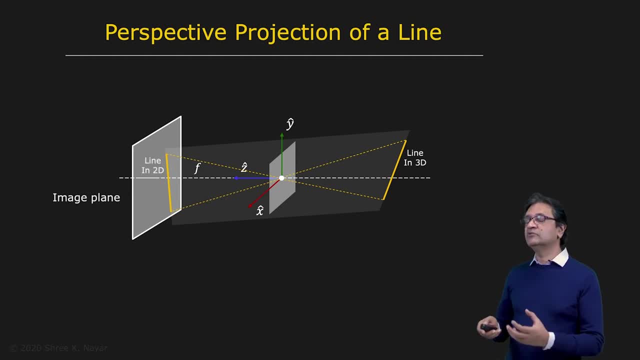 so right here. So in other words, the image of a line in 3D has to be a line in 2D, And this is why you find that in photographs, straight lines in the scene will map to straight lines in the photograph. 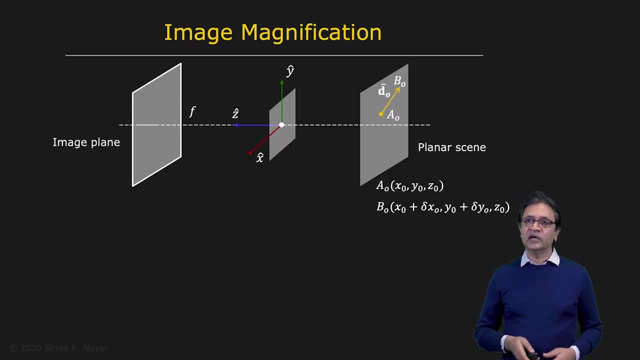 So next we want to talk about image magnification. You have an object of a certain size at a certain distance. What is going to be its size in the image? So for this we're going to use a little segment here: a0,, b0, of length, d0. 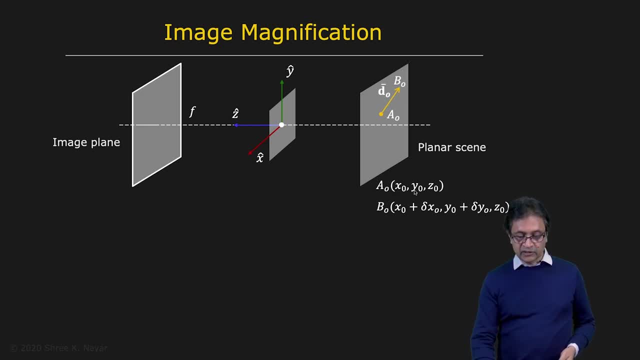 a0 is x0, y0, z0. And b0 is the same coordinates, displaced by x, delta x0 and delta y0. So this segment lies on a plane in the scene that is parallel to the image plane And, of course, it produces an image. 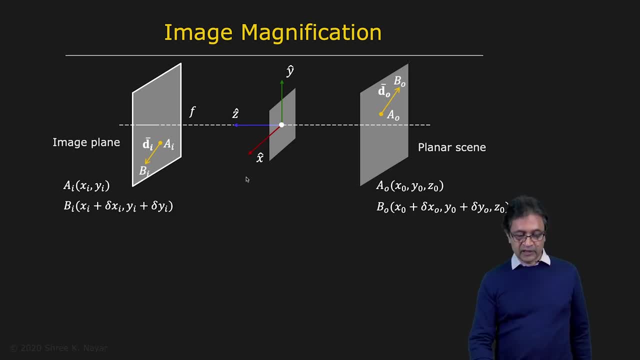 which is another segment, And that segment is ai bi. OK, We want to understand the length of what. the length of the segment ai bi is going to be due to a segment of length d0 in the scene. So the ratio of the length of the segment in the image. 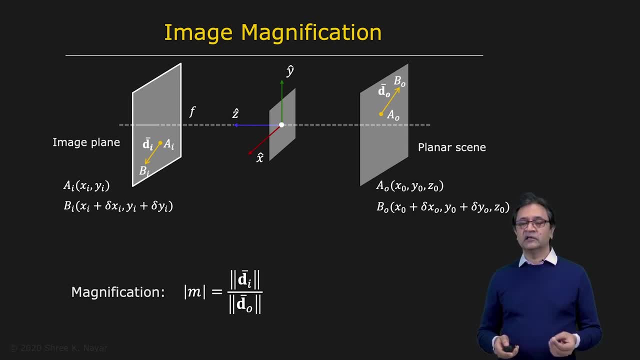 to the length of the segment in the scene is called the magnification, And this, of course, can be written in terms of the displacements delta x0,, delta y0,, delta xi and delta yi as follows. So now we want to substitute for the displacements in the image. 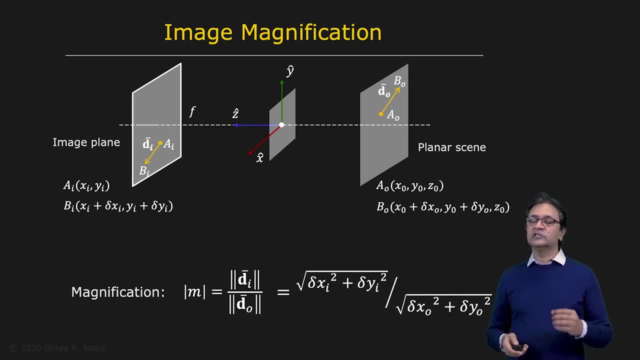 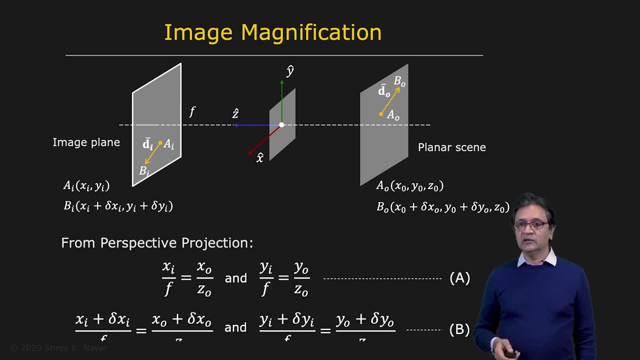 so we can simplify this, And to do that, what we're going to do is apply perspective projection to the point a0 and b0.. In doing so, we are going to get four equations, one for x, one for y, for each one of the two points a and b. 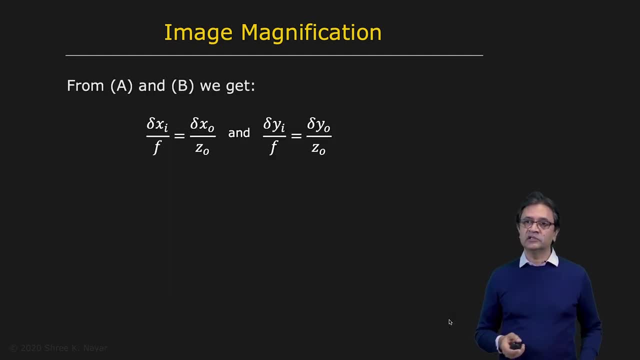 And using these four expressions you end up with a very simple expression for the relation relationship between displacements in the image to the displacements in the scene. And using plugging these back into the equation for magnification, it turns out you get a very simple expression for magnification. 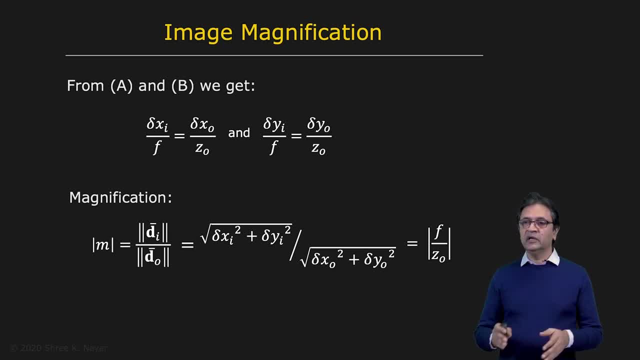 The magnitude of m. the absolute value of m is going to be the absolute value of f. That's the effective focal length divided by z0, which is the depth of the object in the scene. So note that there's z0 in the denominator. 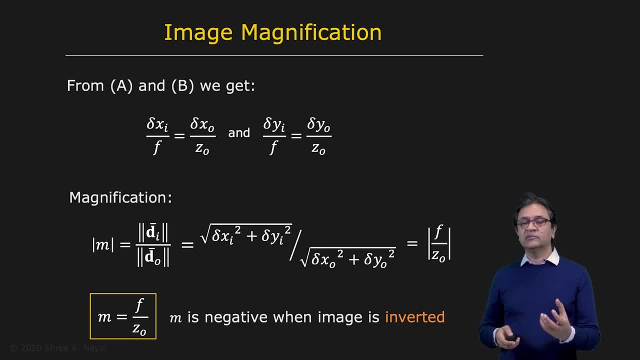 This is a really interesting thing. The size or the magnification of an object in an image is going to be inversely proportional to its distance from the camera And, by the way, the sine of m is going to correspond to whether the image is upright or inverted. 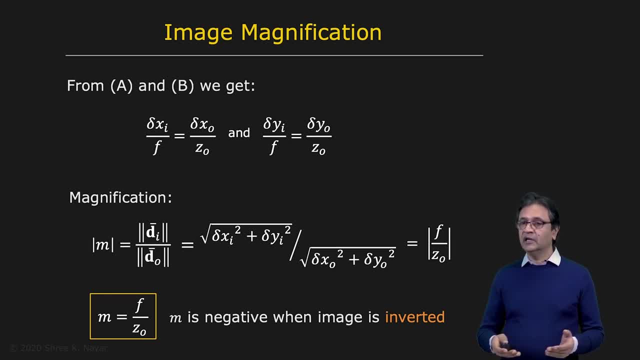 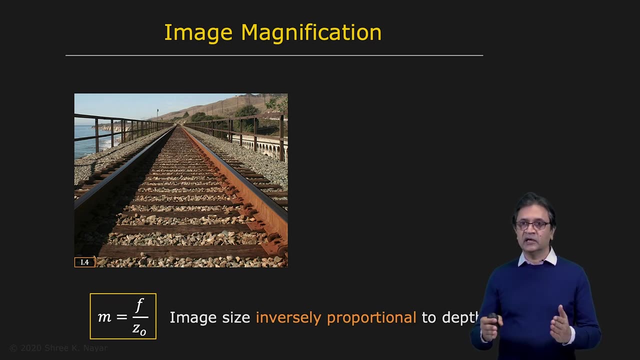 In the case of a pinhole camera of the type that we've just talked about, it's going to be inverted and therefore negative. Now let's take a look at some of the manifestations of image magnification. So here you see, train tracks, two parallel tracks. 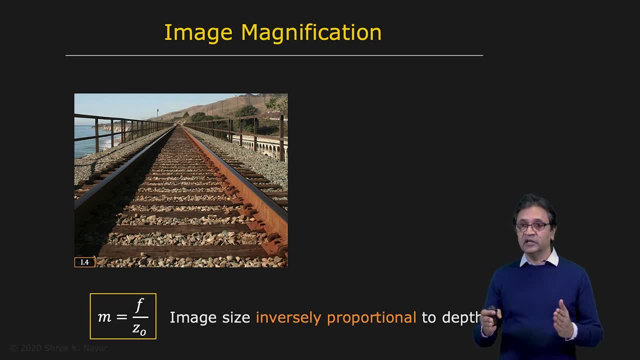 The tracks must be parallel, otherwise the train is going to have a problem, right? We know that these two lines are parallel in 3D And yet in the image they appear to be intersecting or meeting at infinity As you go further and further away in terms of depth. 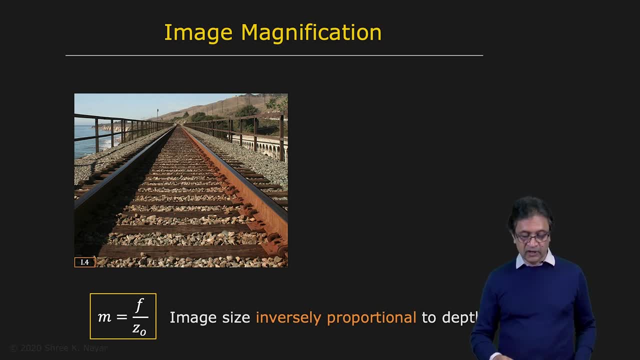 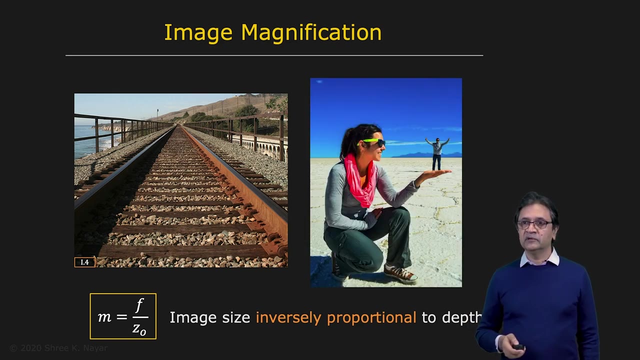 the two lines get parallel. The two lines get closer and closer, And this is because magnification is inversely proportional to distance, z0, depth. So you can actually have some fun with this effect- magnification effect- As a photographer here, you know that these two people are. 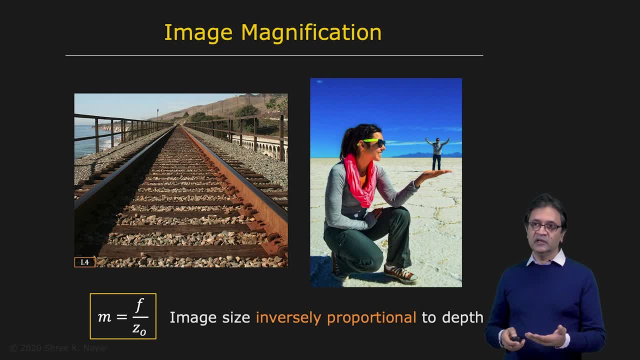 probably roughly the same height And yet the man seems to be standing small enough to be standing on the palm of the woman. A couple of notes About the image, About magnification. The first thing is that the magnification of an object 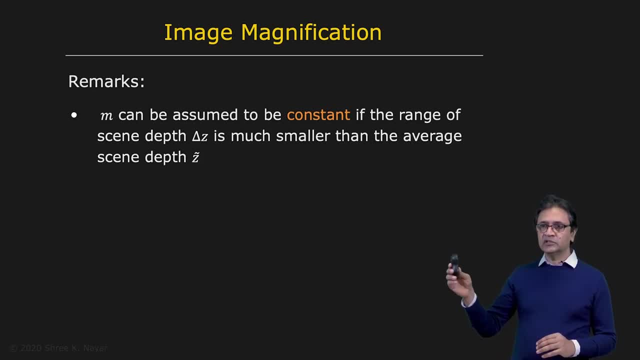 can be assumed to be constant if the object is small compared to its distance from the camera. So, if this is the object, its range of depth values is small compared to its distance from the camera. Let's assume that my eye is the camera. 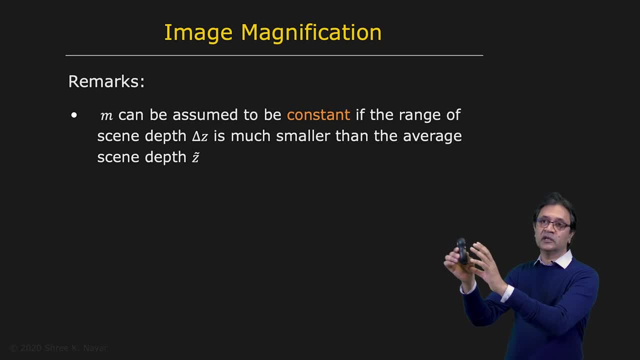 Then you can assume that the entire object is being subjected to the same magnification. This is an interesting thing, because there is a reason why in selfies, say, for instance, your nose tends to look much larger than the rest of your face, And the reason is that the nose, in the case of a selfie, 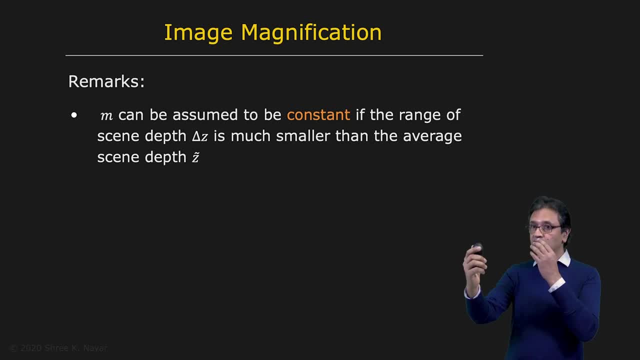 the camera is actually quite close to your face And the nose is closer to the camera than your ears or your eyes And therefore appears, tends to be magnified a lot more than the rest of your face, And then you can also now talk about. 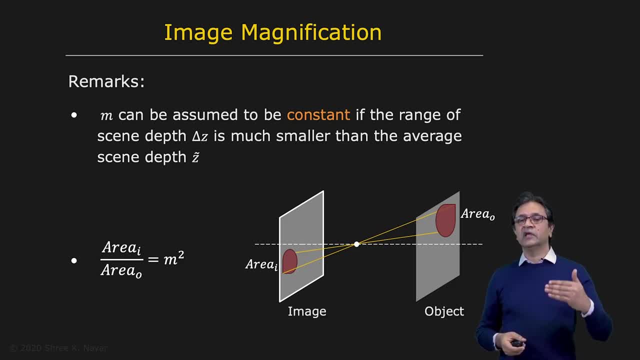 once you have magnification, you can talk about the ratio of the area of an object in the image to its area in the scene, And that would be m squared. Now let's talk about an interesting manifestation of perspective projection, And that's the vanishing point. 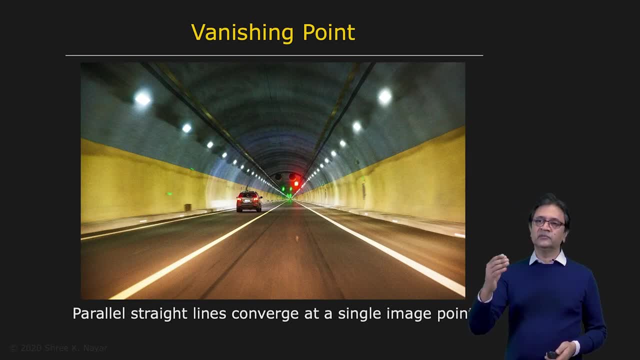 So in this picture, this is a picture of a tunnel. Let's assume for a minute that the tunnel is a straight tunnel And the tunnel has a lot of lines. These are lines in 3D- 3D. For instance, the white lane lines right here. 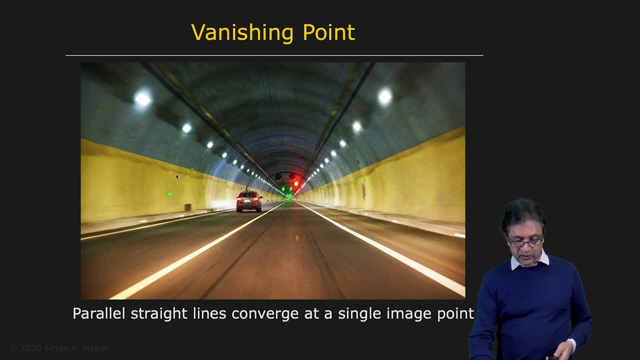 and the edge of the yellow bands. The two edges of the yellow bands are also straight lines. In fact, the track of lights that you see up also lie up here lie on a line, as well as these dark lines right here. We can assume that all of these lines are parallel in 3D. 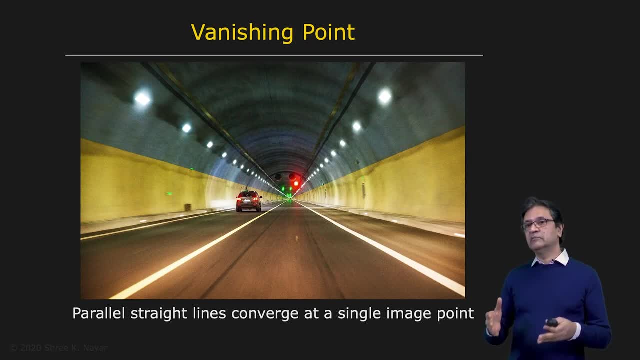 because it's a tunnel And yet all of them seem to be emerging. But what we can do is we can't see them from a single point in the image and that point is called the vanishing point. So if you have a set of parallel lines in 3D, 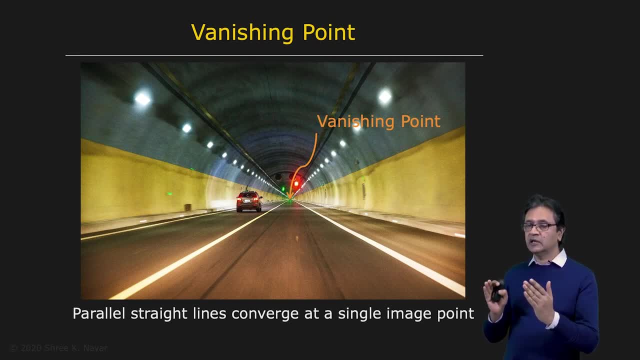 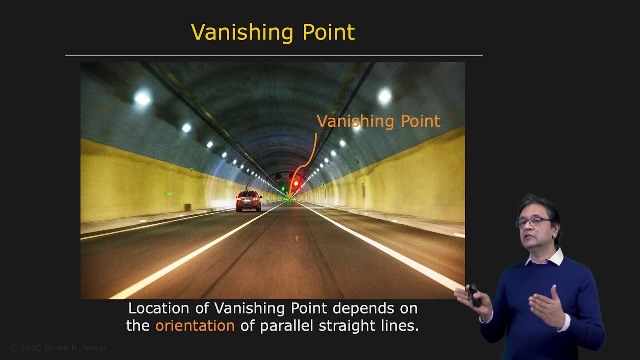 they end up producing. It doesn't matter how many parallel lines, They end up sharing a single vanishing point. They seem to be converging at the single point in the image, And the location of this vanishing point depends on the orientation of these parallel lines in 3D. 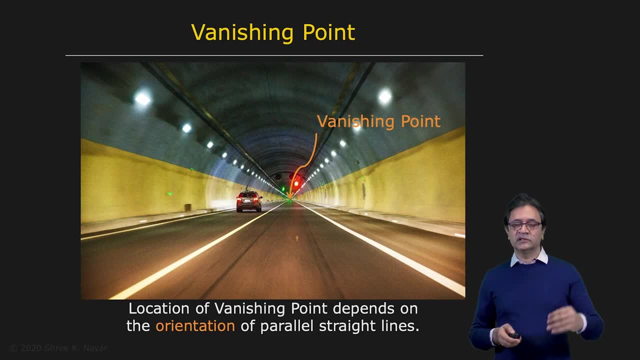 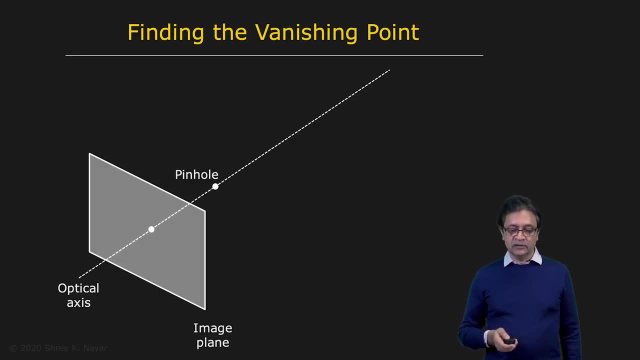 So how do we figure out, given a set of parallel lines in 3D, where the vanishing point is going to end up for that set of lines? So here is a very simple way one can figure this out, a very intuitive way to do it. 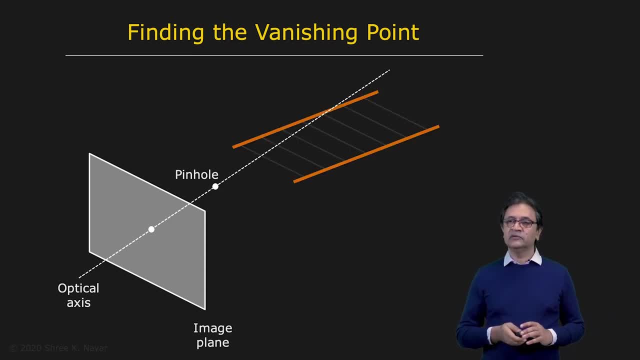 So assume that you have these two parallel lines And we want to find the vanishing point corresponding to these two lines. Can you think for a minute how you might do this? Well, remember, all parallel lines in 3D share the same vanishing point. 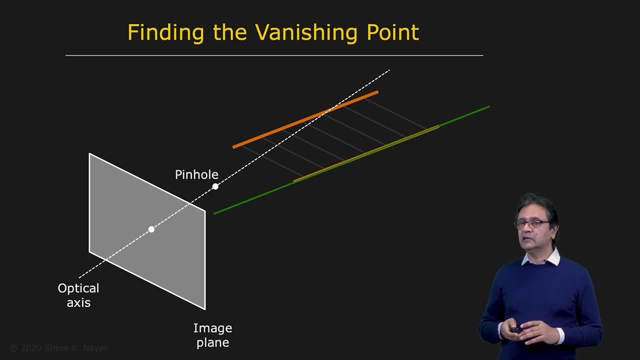 So what you need to do is to construct a line that is parallel to these two lines, that passes through the pinhole, And wherever that line pierces the image is the vanishing point corresponding to the set of parallel lines in 3D. So how do we find this? 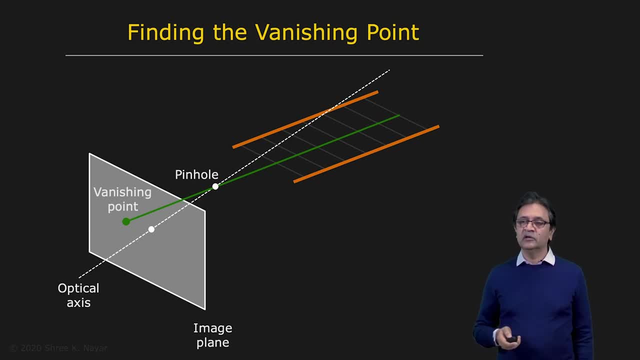 Well, that's very straightforward, given that we know perspective projection. we first define the direction of the set of parallel lines in 3D That's given by the vector Lx, Ly, Lz- And then we create a point which is in that direction. 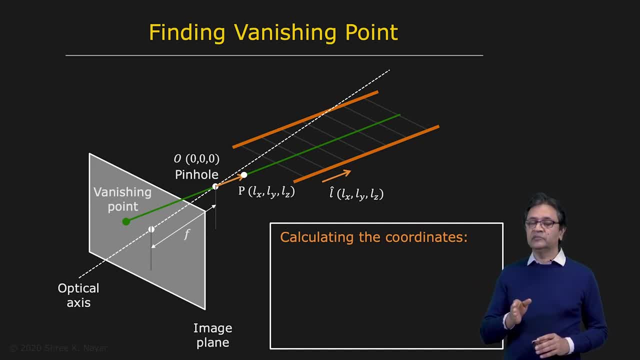 the point P in that direction from the pinhole of the camera. So that's the point P that you see right there. And now you simply prospectively project that point into the image using perspective projection equations And you get the location of the vanishing point. 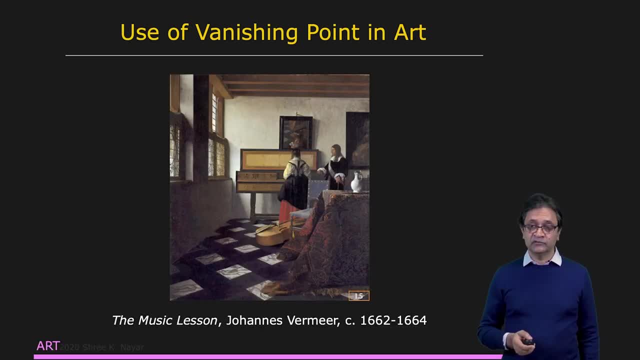 So the vanishing point is a concept that artists have used extensively. Here is an example: Johannes Vermeer painted The Music Lesson, very famous painting by this Dutch artist. And in this scene here you have a lot of parallel lines or sets of parallel lines. 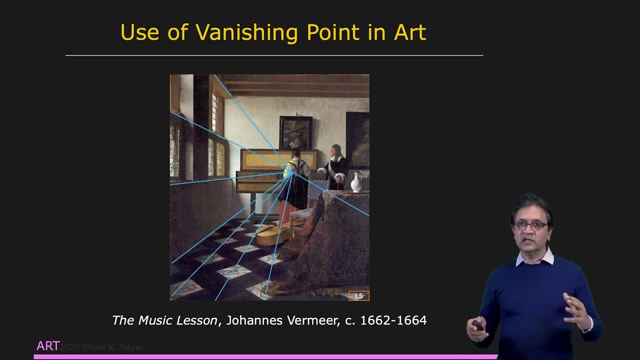 But let's take a look at this set right here. You see that this set of parallel lines ends up converging at this point. This is the vanishing point right here, And what Vermeer has done is place what he considers to be the most important object or activity. 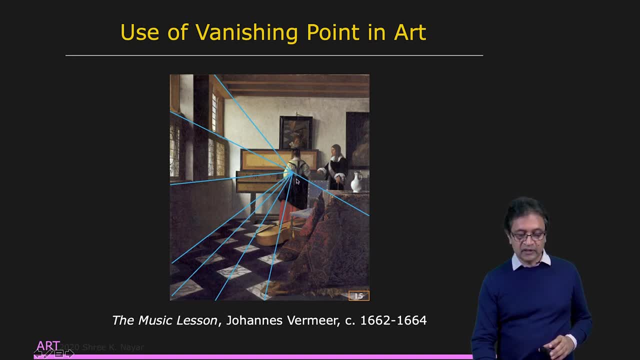 exactly at that place. In this particular case it sits at the elbow or close to the elbow of the student who's playing the piano. He wants to draw your attention to that activity. So a lot of our work is done in this way. 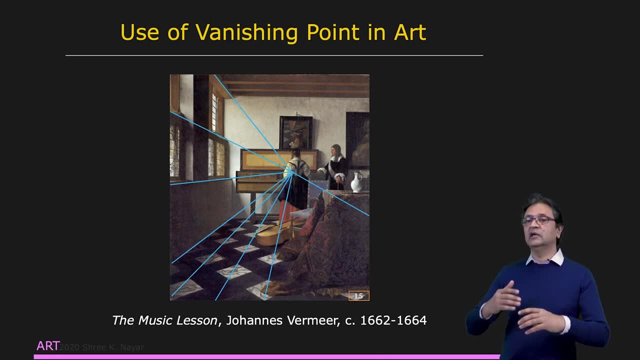 So a lot of artists figured out early on that humans in any three-dimensional scene, in any photograph, tend to be drawn to vanishing point, especially dominant vanishing points that are created by large numbers of parallel lines, And so they played this trick of placing 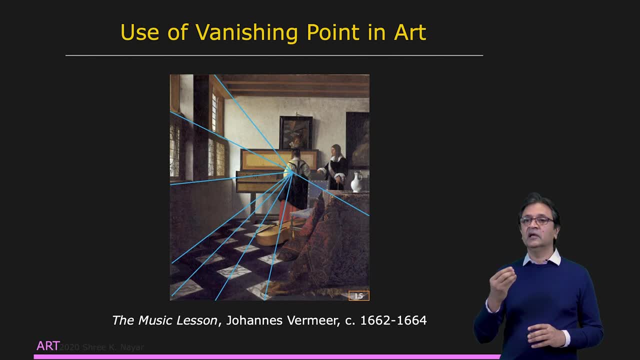 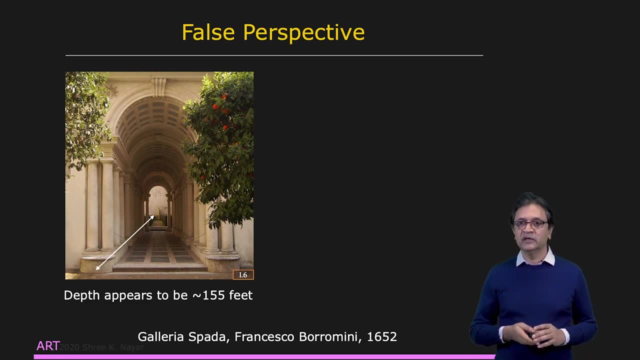 the most important subject or activity at those points. Here's another interesting concept, which is called false perspective. This is Galleria Spada by Francesco Borromini. It's a beautiful little gallery in Rome. I've had the good fortune of visiting it. 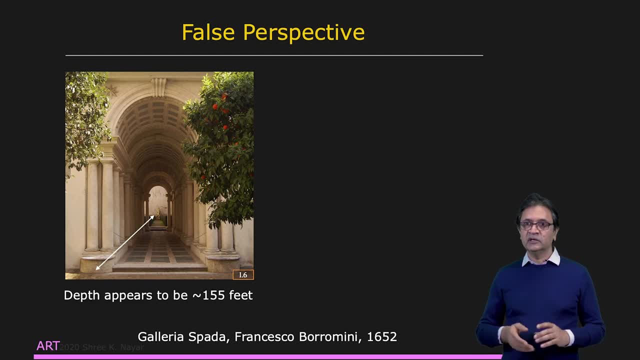 and it's a really compelling effect. So what you see here is a archway or a little bit of a hallway, And at the end of the hallway you have the sculpture, And when you stand in front of the hallway you get the impression that the sculpture is roughly 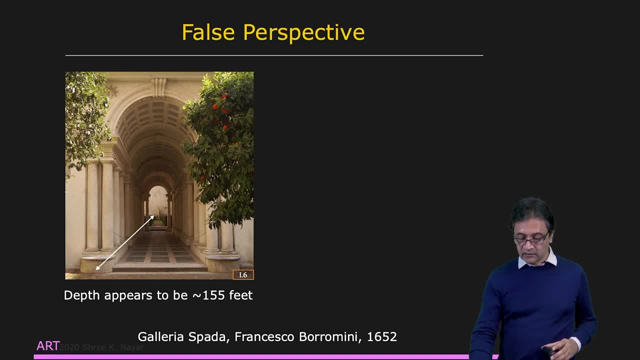 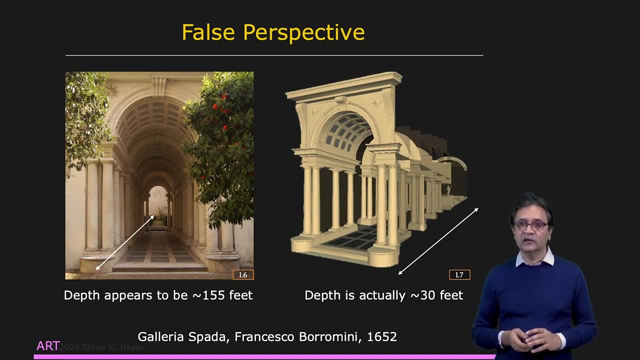 150 feet away from you. It turns out that the sculpture is only 30 feet away from you, And the reason you have this very compelling effect or illusion is because the pillars of the archway are actually getting smaller with distance away from the observer. 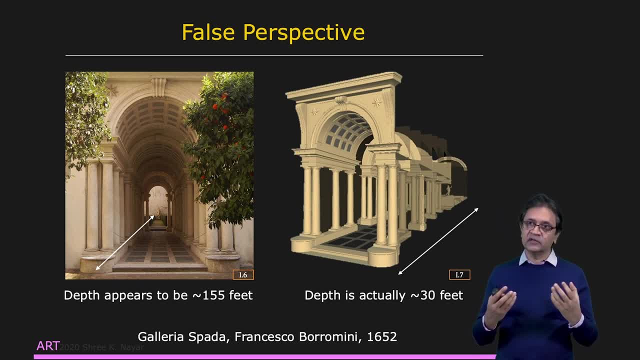 So it's a tapered archway And this creates this effect of false perspective which forces you to believe, leads you to believe, that the object at the end of the hallway is much further away. Then it actually is OK. So we talked about the pinhole and how. 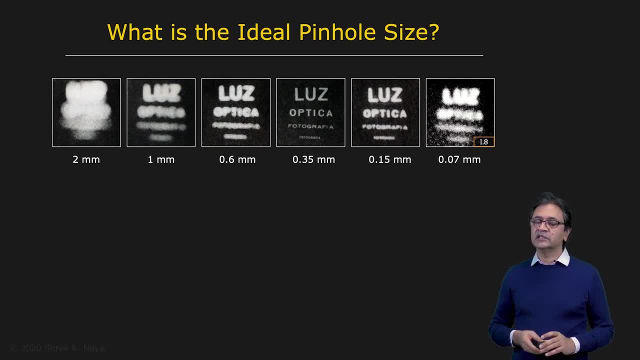 it can be used to create images. But one thing we sort of set aside is the size of the pinhole. What should the size of the pinhole be? Well, we said, it's a point, It's a tiny little hole. And that makes a lot of sense, because the tinier the hole, 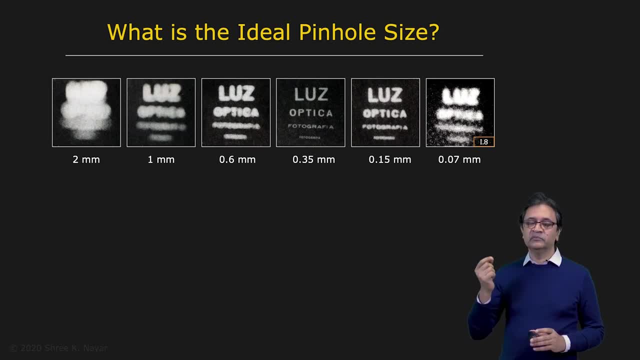 obviously you're going to have a thinner, better defined ray going through, But not quite. If you look here You have the size of the pinhole used to take a set of images, And we start with the largest size, 2 millimeters, here. 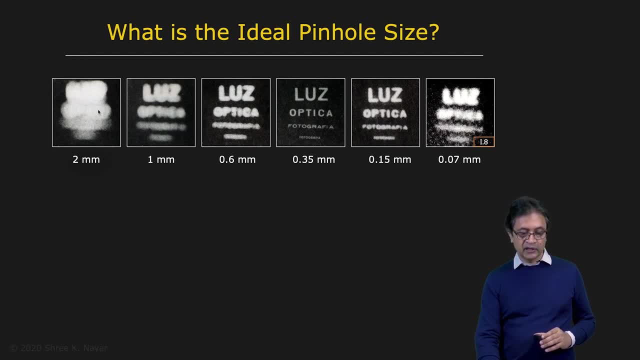 And because it's fairly large, you're going to get a lot of blurring in the image, Because from each point in the scene, as you can imagine, you don't get a single point in the image, But you'd rather end up getting a bundle of rays. 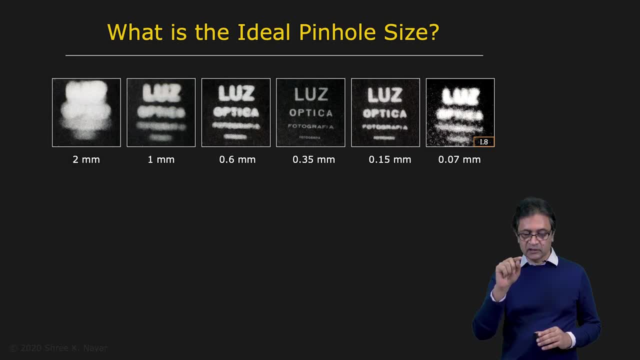 going through, which creates a distribution of light in a circular region. So you get a blurry image. As you start making the pinhole smaller- 1 millimeter- you see that it gets sharper- 0.6.. And then finally, at 0.35, you get a very sharp image. 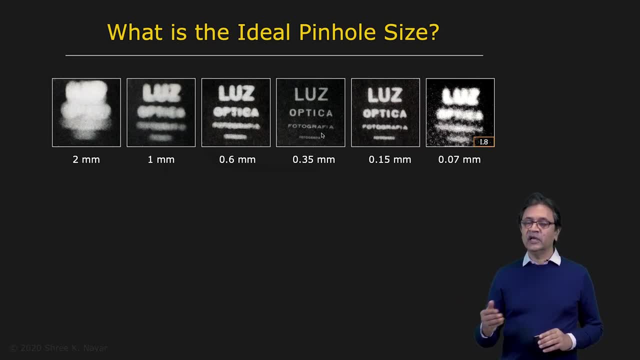 But here's the interesting thing: You go smaller, You make the pinhole even smaller. Actually, the image starts getting blurrier again. So here you see, at 0.15, it gets a little bit blurry. 0.07, it's even blurrier. 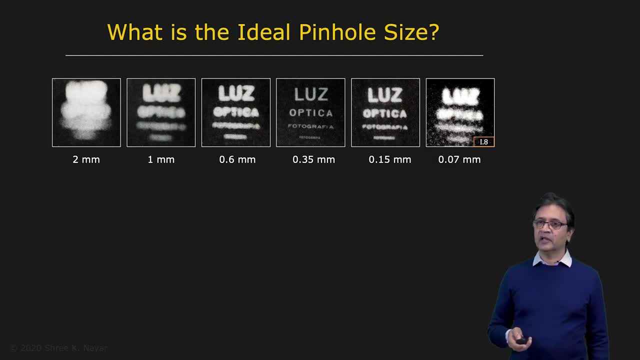 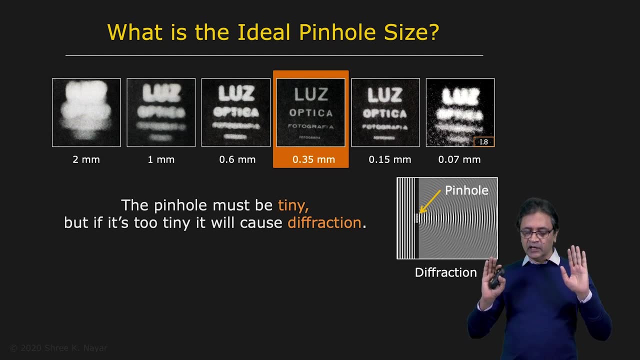 So why does this happen? This is because of an effect in wave optics called diffraction. So it turns out that if you have any opening and you have a light wave that's passing through this opening, there's going to be a bending of these light waves. 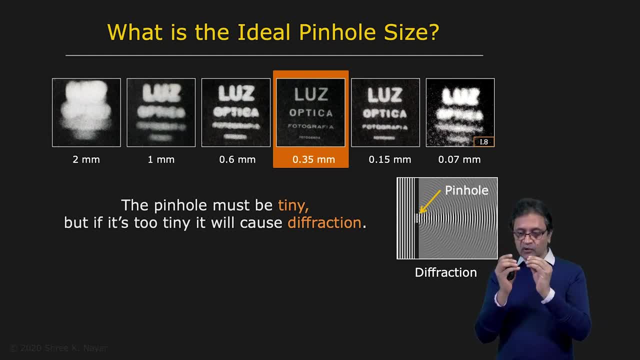 at the edge of the periphery of the opening, And the smaller the opening gets, there's going to be more the effect of the bending than the light actually passing through, And so you get severe bending as you get too small. So then the question is: how do you? 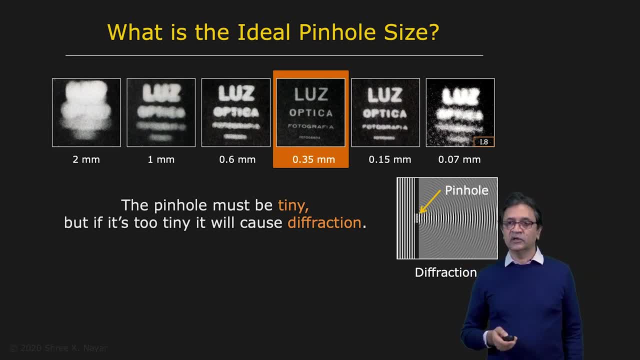 measure the effect of focal length and the wavelength of light. And the question is: what is the ideal size of the pinhole? Well, you can calculate this And it turns out to be: the diameter of the pinhole should be two times, roughly two times. 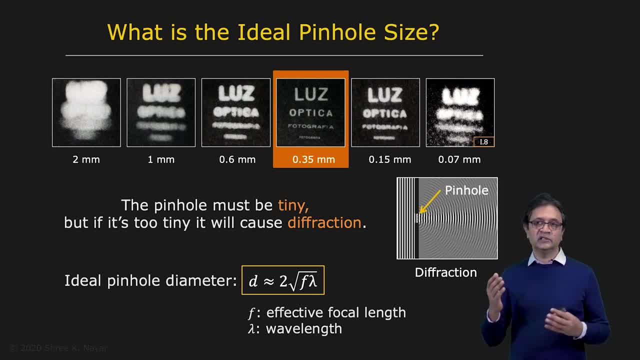 square root of the product, of the effective focal length and the wavelength of light. So in our case, if you're interested in visible light images, the wavelength lies somewhere between 400 nanometers and 700 nanometers, So let's just pick the average. 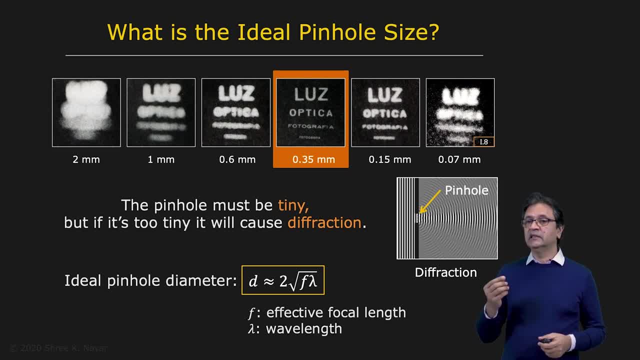 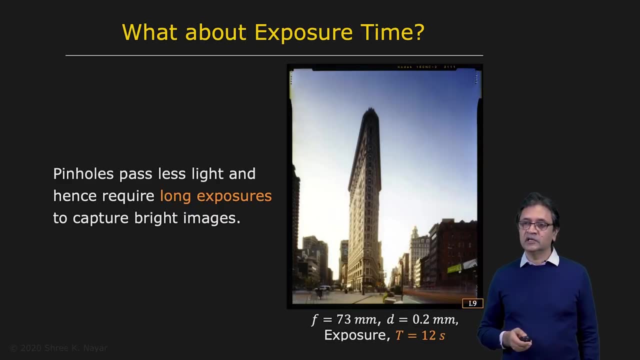 And then you would plug in the effective focal length And then you would get the ideal, or close to ideal, pinhole diameter, And that's what you should be using to capture your images. So if you use the ideal pinhole size, you can get some stunning images. 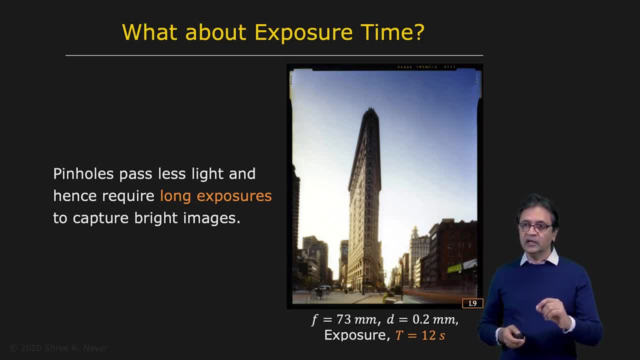 So here's an image of the Flatiron Building in New York, And one of the interesting things you notice is that the image is pretty much focused everywhere. So pinhole cameras- well-designed pinhole cameras- tend to create these sort of all-focused, focused.